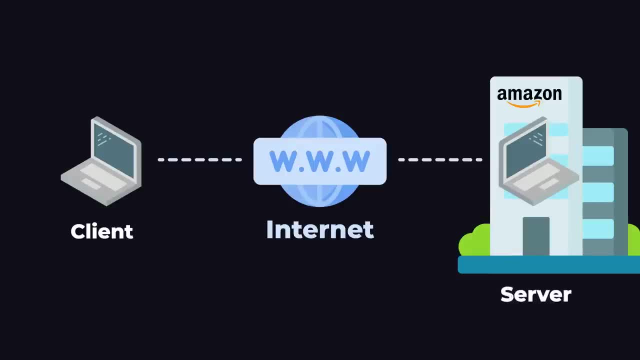 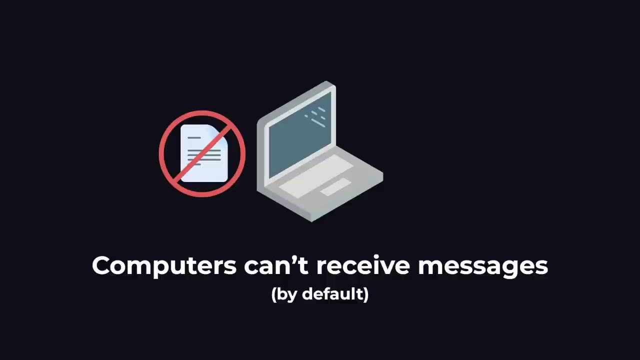 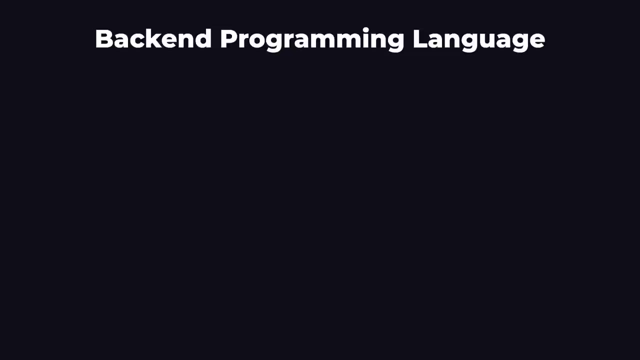 and the computer that is receiving the message is called the server. But before this happens, computers can't receive messages from the internet by default. We have to program them to be able to receive messages. To do that we need a back-end programming language. Almost every programming. 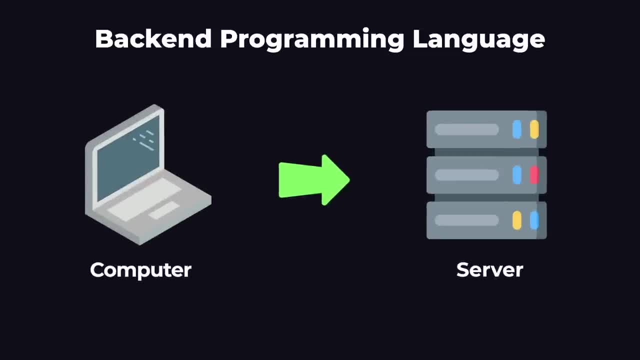 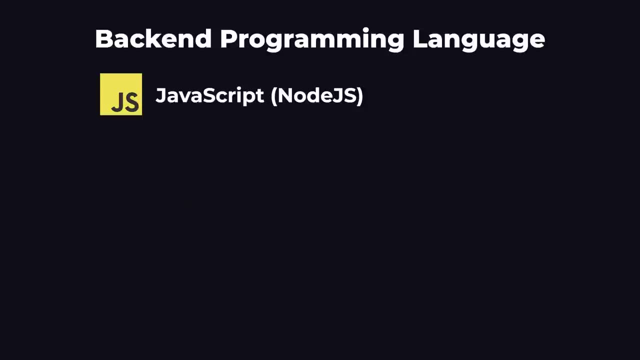 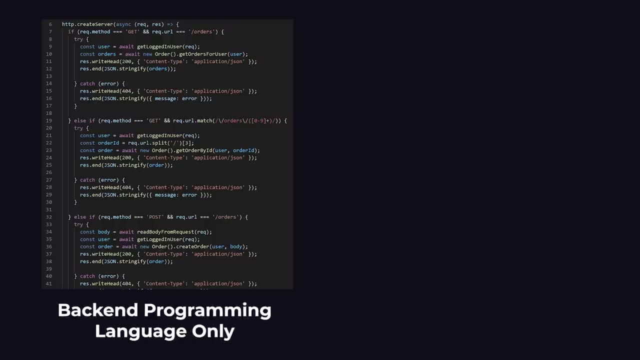 language has a feature that turns a computer into a server and allows it to receive messages. Popular back-end programming languages are javascript, sometimes called nodejs, python, ruby and java. However, using a back-end programming language by itself is actually really difficult and requires a huge amount of code. So there are 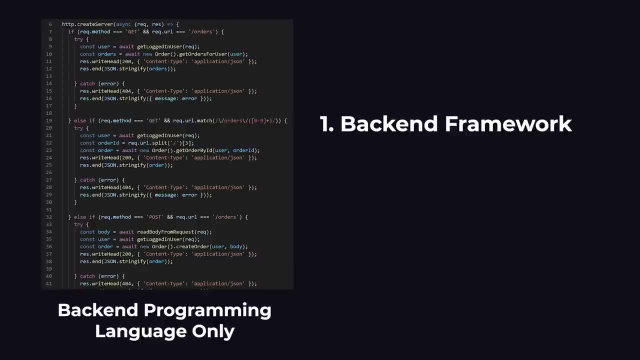 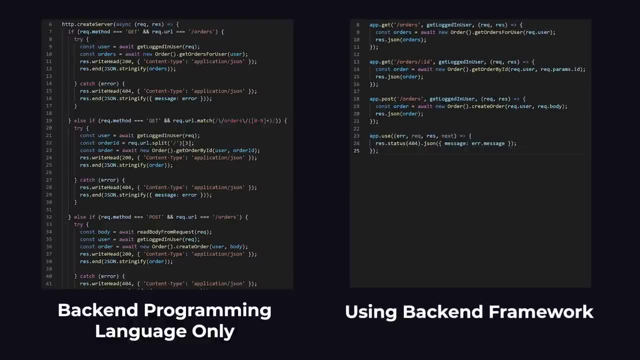 two tools that we use to help with this: a back-end framework and a package manager. A back-end framework helps us create a server much easier and with a lot less code. Each back-end programming language has a few different frameworks to choose from, but the most popular ones are: 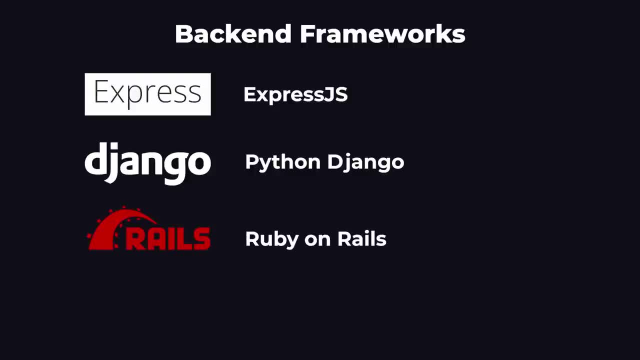 expressjs for javascript, python, django, ruby on rails and javaspring. In the back-end we also use a lot of code that other people have written, called packages, to do common tasks like doing calculations, talking to a database. 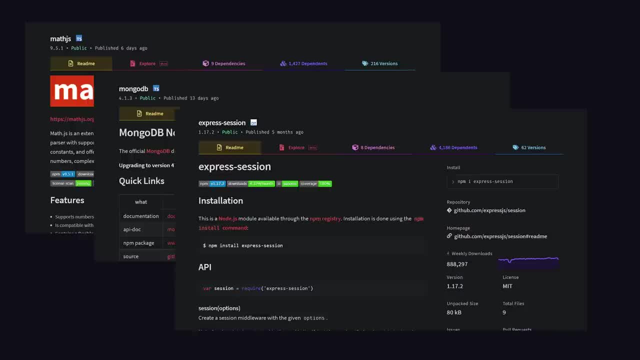 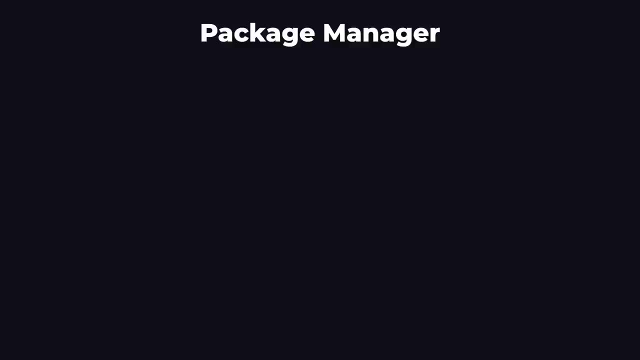 and setting up user login and authentication. We typically use a lot of packages in our back-end and in order to install and manage all these packages, we use something called a package manager. Each language has its own package manager, and the popular ones are npm for javascript, pip for python, bundler for ruby and maven for java. 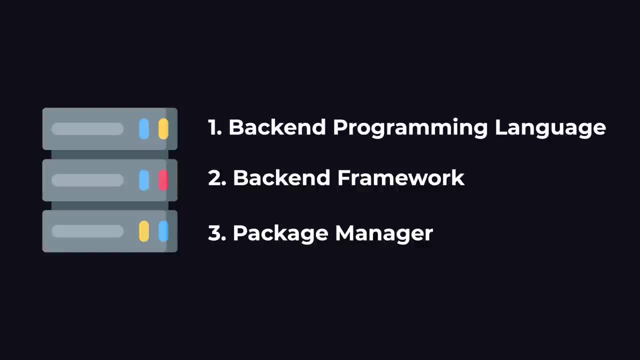 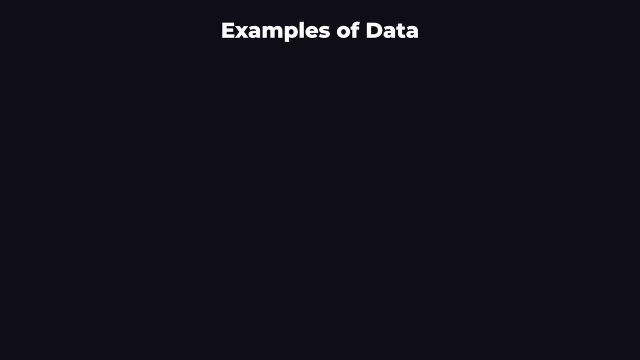 These are all the technologies we need to create our back-end server. The next problem we have is we need somewhere to save the data for our website. Going back to our Amazon example, data could mean our user data, like the login information. 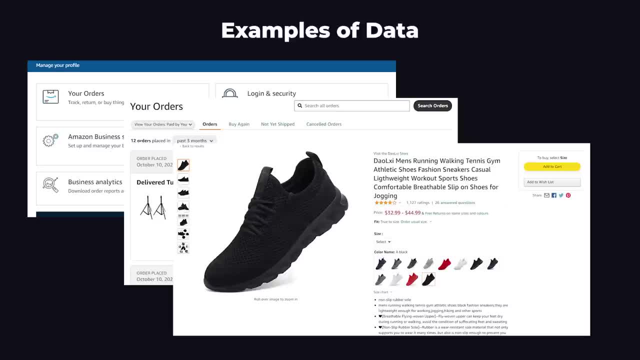 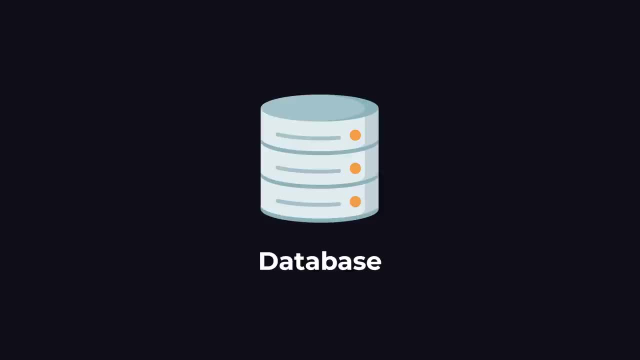 order history, as well as data for all the products that are being sold on Amazon: the descriptions, the ratings and the reviews. To do this, we use a database. A database helps us store and manage data. It's just a piece of. 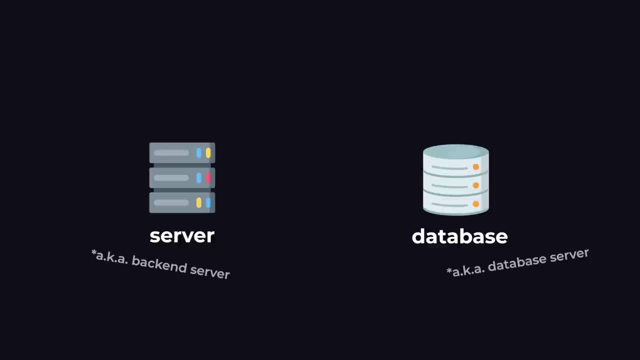 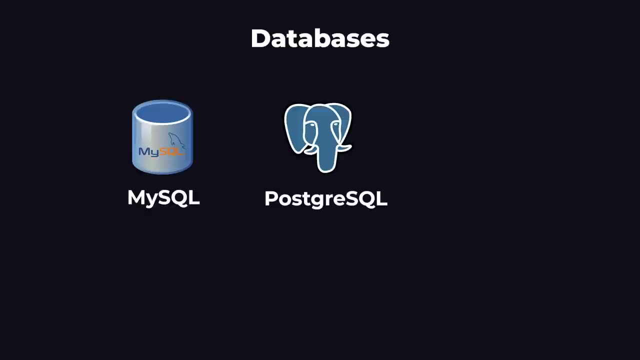 software that usually runs on a different computer and we have to do some setup so that our back-end can communicate with the database. The most popular databases are MySQL, Postgres and MongoDB. Alright, so if you're just starting out, this is basically all you need for. 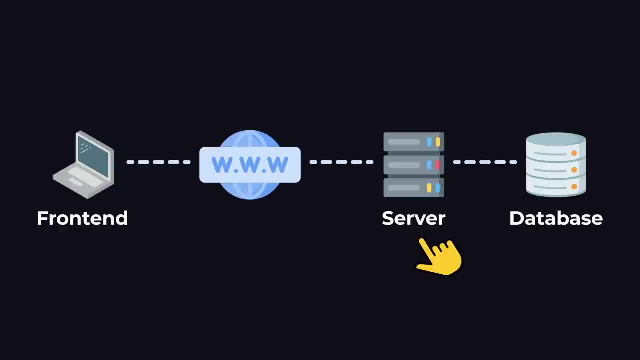 the back-end. You can build most of your projects with just a server and a database. For example, here's how our Amazon scenario could work: When the customer places an order in the front-end, the front-end sends a message containing the order to the back-end. The back-end then saves the order to a database. 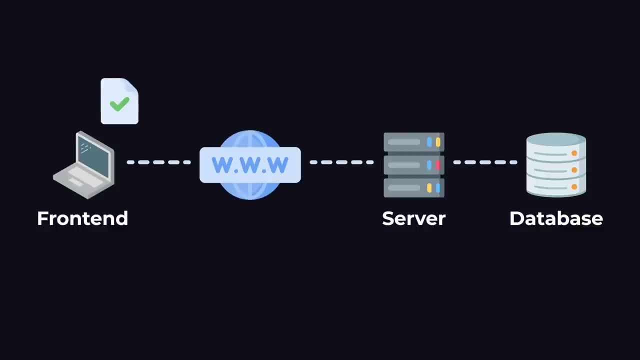 and sends back a message to the front-end confirming that the order was created. The message that the front-end sends to the back-end is known as a request and the message that the back-end sends back is known as a response. This is called a request. 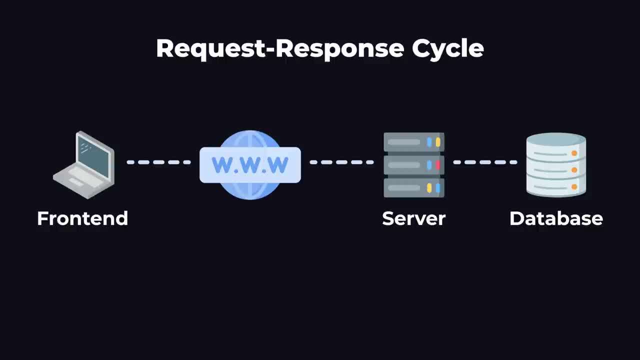 response cycle, and this is generally how web applications work. Here's another example. Let's say that you're in the Amazon warehouse. The warehouse might have a different front-end that sends a request to the back-end to get our order. The back-end then gets our order. 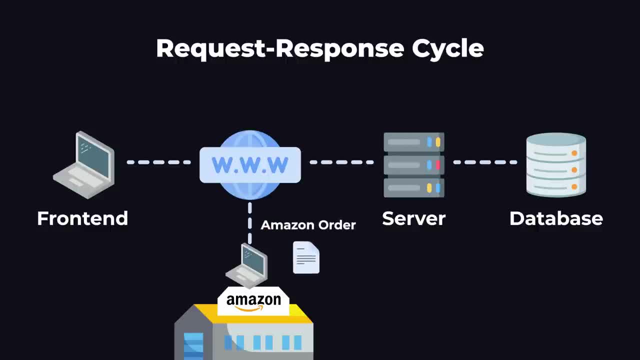 from the database and sends it back to the warehouse front-end, and then they go ahead and prepare our order. Now that we've seen the overall flow, we're going to dive deeper and take a look at what's inside a request. Here's a simplified example of a request to create an. 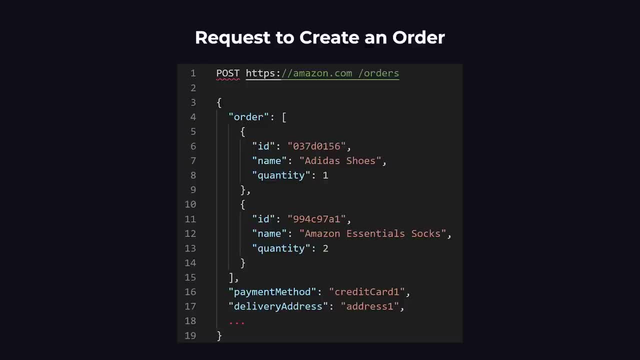 Amazon order. If we read over it, we can see that it's actually really easy to understand. We have the items that we ordered, the quantities and some other information about our Amazon order. At the top we have the type of the request, the domain name and the URL path. This describes. 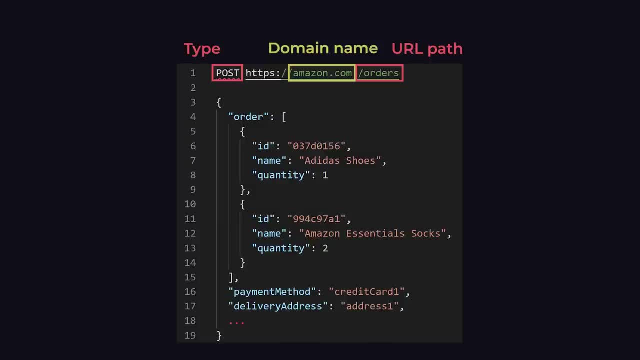 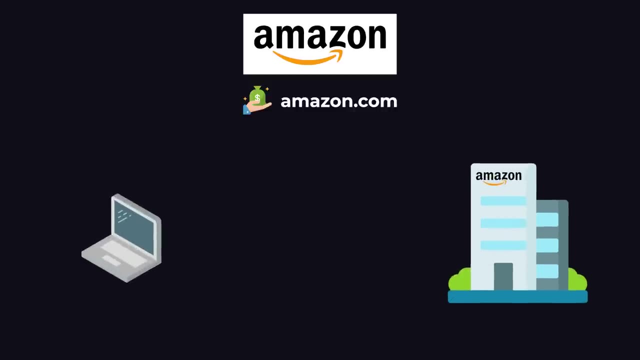 where this request is going and what type of request this is. First of all, Amazon. the company has bought the domain name amazoncom and they configured it so that any requests going to amazoncom will be redirected to that server in their office building. So that's why. 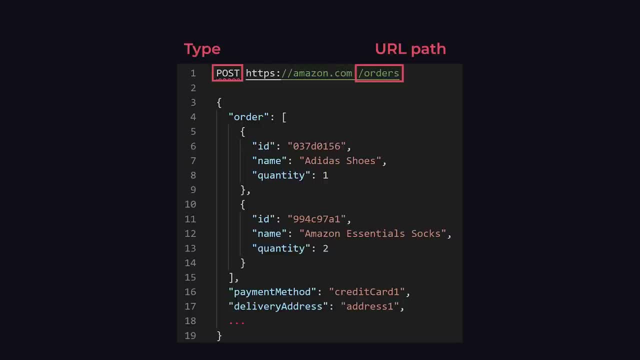 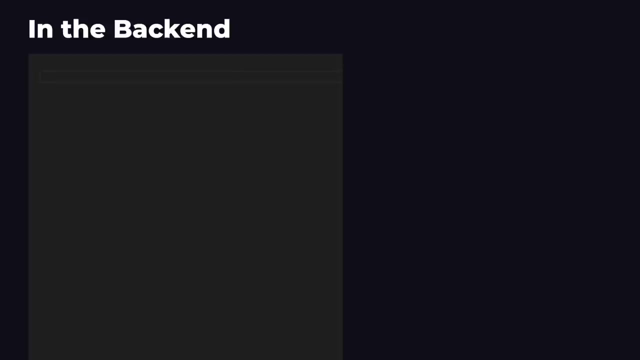 we're sending this request to amazoncom. The type and the URL path identify what kind of request this is. So in this example, this is a POST request to slash orders In the back-end. we use our programming language and back-end framework to define what types of requests are allowed and how. 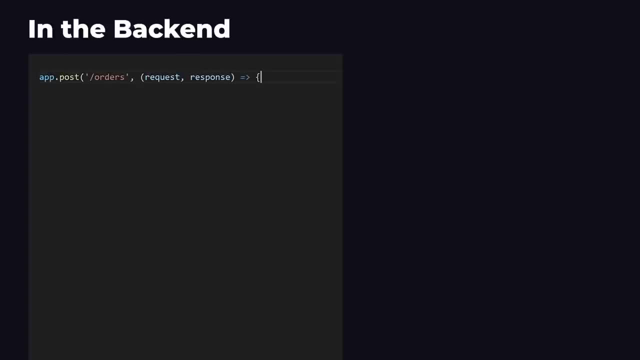 we should handle these requests. For example, we can allow a POST slash orders request and whenever we get a POST slash orders request, we will create an order using our programming language and save it to our domain. We can also allow a GET slash order request and in this case we will retrieve the order history. 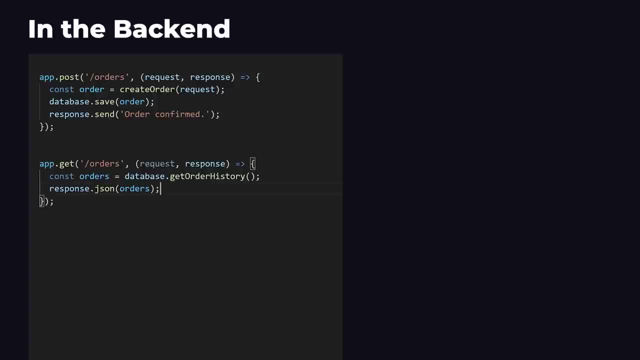 from the database and send it back as a response. Another example is a DELETE slash order request, where we will cancel the order. So this list of all the different types of requests that the back-end allows is called an API- Application Programming Interface. The API is one of the most important. 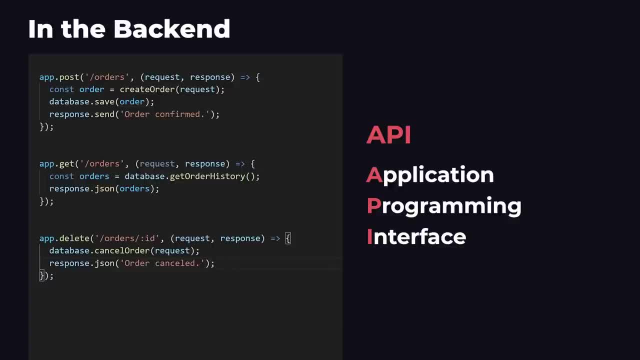 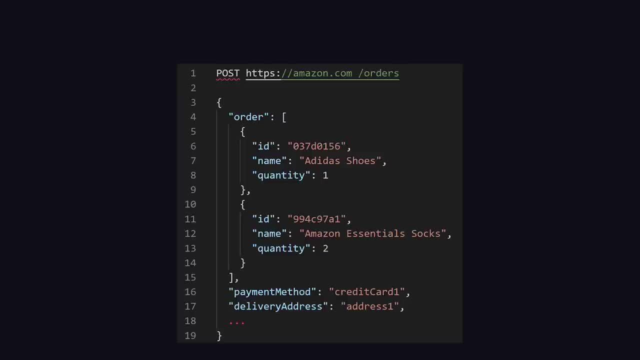 concepts in back-end programming. If you send a request that is not allowed by the API, the back-end will respond with an error. So we mentioned earlier that we can identify requests using a type and a URL path. There are several types we can choose from, such as POST, GET, PUT and DELETE. 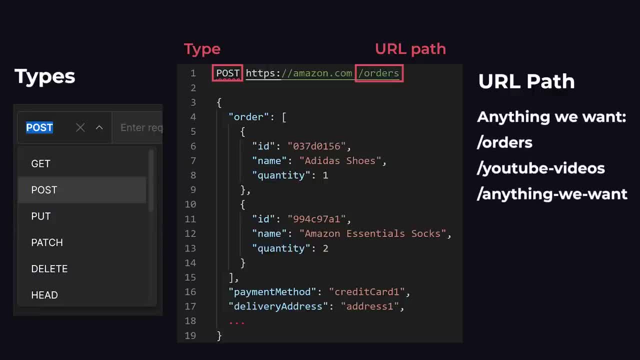 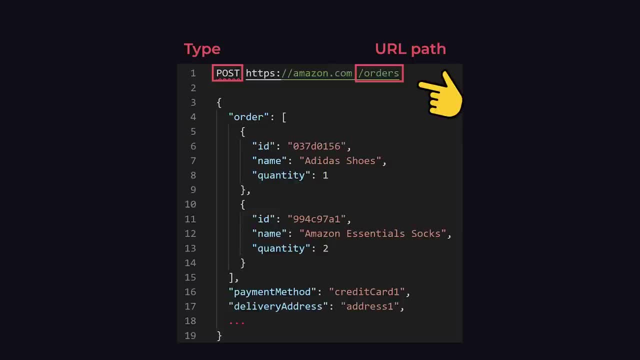 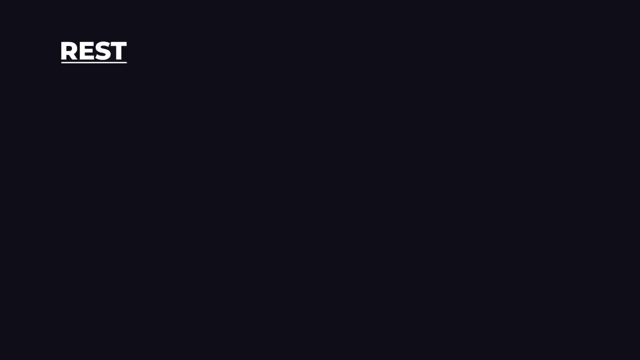 and the URL path can be anything we want. So why, in this example, did we choose POST slash orders? This is just a naming convention for our requests, and this naming convention is called REST- Representational State Transfer. In REST, the type of the request has a special meaning. 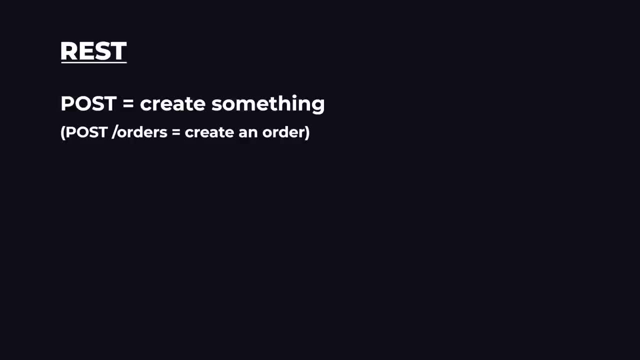 so POST is the name of the request, and the type of the request has a special meaning. so POST is the name of the request. POST means to create something and in this case, POST slash orders means to create an order. GET means to get something and DELETE means to delete something, and so on. 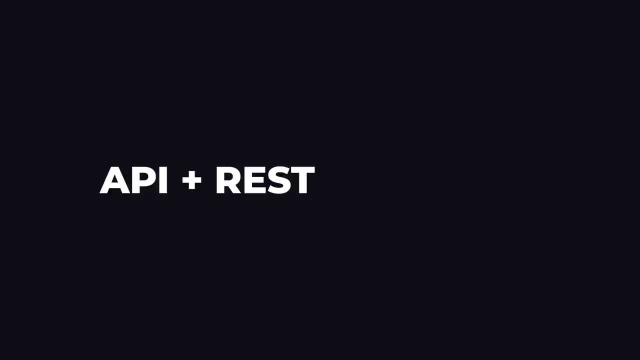 An API that uses the REST naming convention is called a REST API. REST is the most common convention that we use for our APIs, but there are several other conventions that we could use. One of them is called GraphQL, which uses POST slash GraphQL for all of our requests. 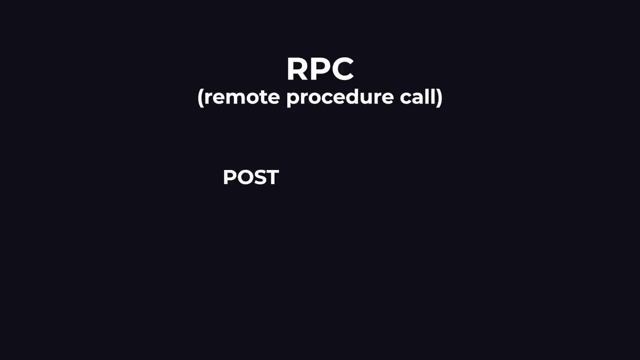 and another one is called RPC, which uses POST and a more detailed URL path like POST slash- CREATE ORDER or POST slash- GET ORDER HISTORY. So that is what a request is, what an API is and what REST means. Now let's talk about. 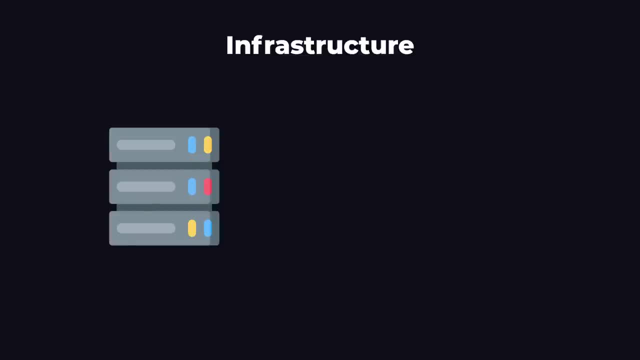 infrastructure. Nowadays, instead of companies purchasing their own computers to run their websites, they rent computers from a cloud computing company. The biggest cloud computing companies are AWS, Amazon Web Services, GCP, Google Cloud and Microsoft Office. The biggest cloud computing companies are AWS, Amazon Web Services, GCP, Google Cloud and Microsoft Office. 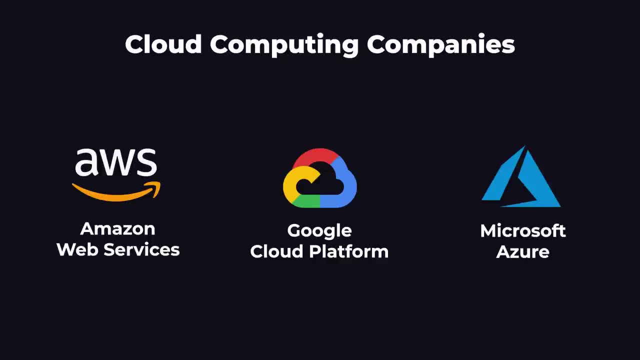 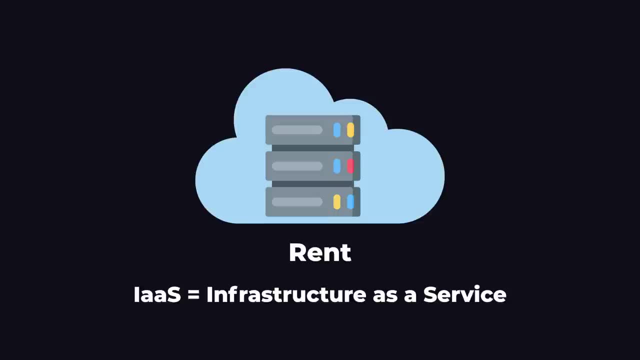 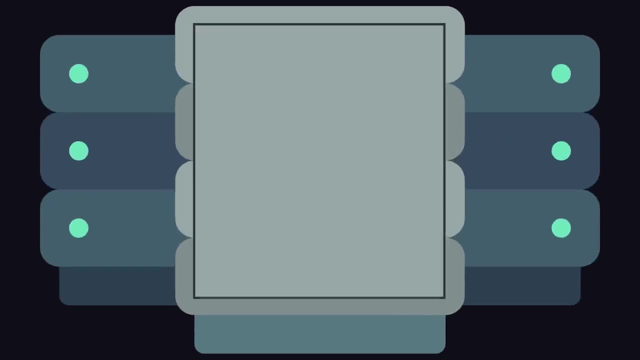 The biggest cloud computing companies are AWS, Amazon Web Services, GCP, Google Cloud and Microsoft Office. The basic idea of cloud computing is you're renting a bunch of computers- This is also known as IaaS infrastructure- as a service. Behind the scenes, AWS has a giant, powerful computer and inside its software it's running. 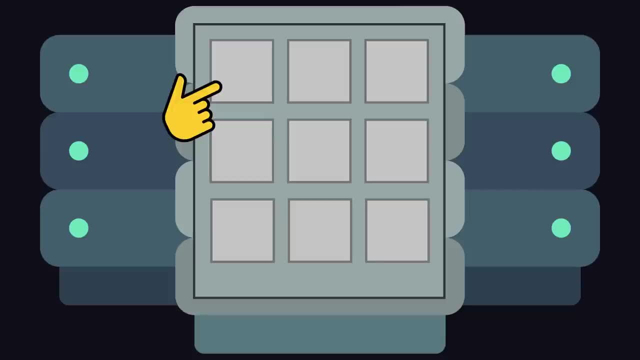 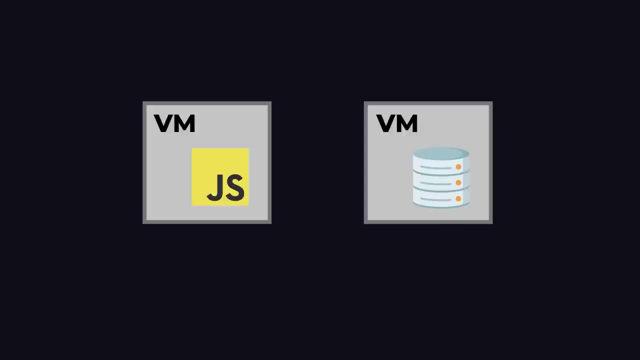 many smaller computers and we're actually renting one of these smaller computers. And these smaller computers only exist in the software, so we call them virtual machines or VMs. So to run our website we rent a VM from AWS to run our backend and we also rent another VM to run our database. 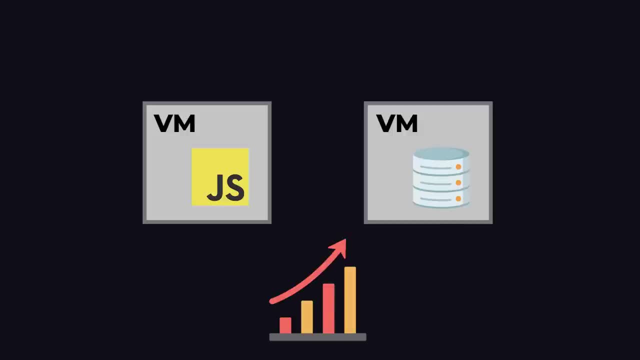 Another problem we have to solve is what if our website gets really popular during the holiday season and we start getting a lot of requests and internet traffic that our server can't handle. With cloud computing, we can set up multiple VMs running the same backend code and then set up a. 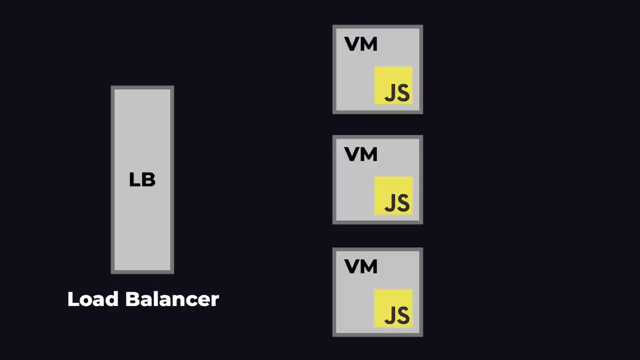 special VM in front of these, called a load balancer, And the load balancer will distribute requests evenly across our VMs. And the load balancer will distribute requests evenly across our VMs. Once the holiday season is over, we can just shut off our VMs when we don't need them. 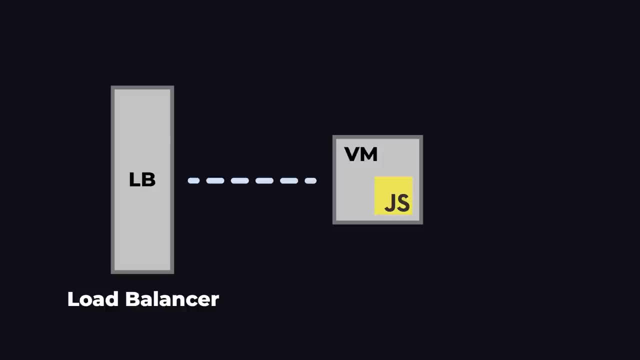 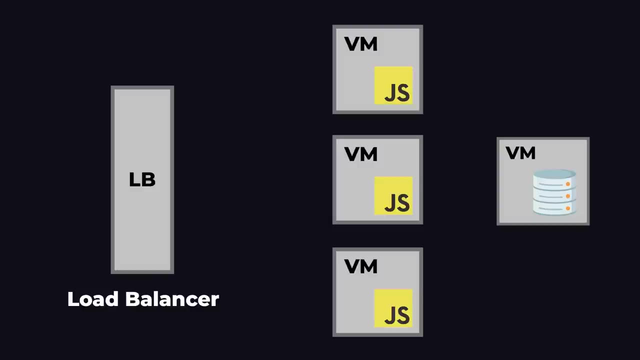 This is a lot easier than having to buy physical computers where, if the holiday season is over, you still have the physical computers that you paid for. But we still have another problem. We now have a lot of VMs that we need to create and set up. 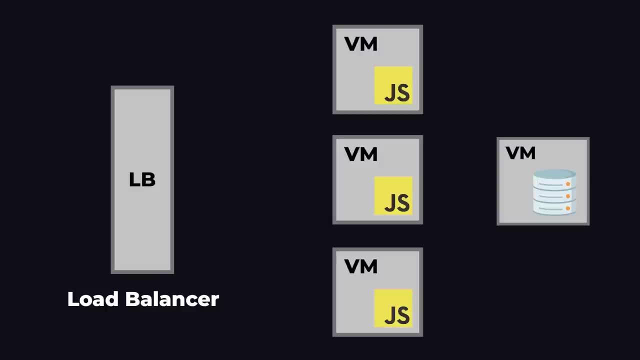 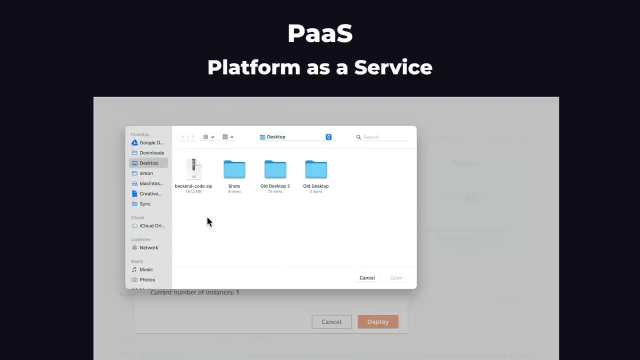 and it takes a lot of time and effort. Cloud computing companies offer another service called a PaaS, a platform as a service. A PaaS just lets us upload our backend code. it will set up all the VMs, including the load balancer, and integrate everything for us. The three most: 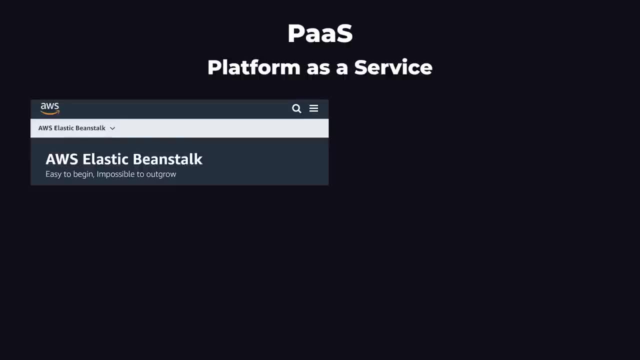 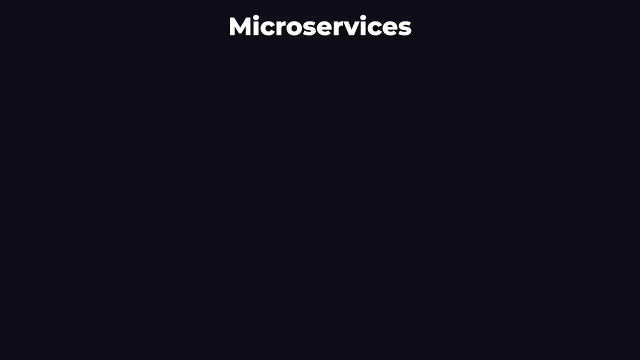 popular PaaS are Elastic Beanstalk for AWS, App Engine for GCP and App Service for Microsoft Azure. The next concept we're going to look at is microservices. For our Amazon example, let's say that our backend contains code that saves an order to the database charges the user's credit card. 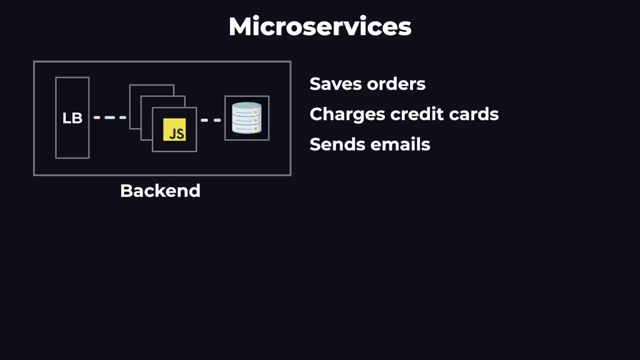 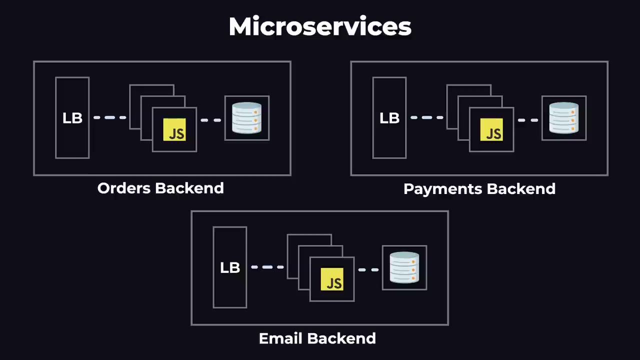 and sends an email confirmation. In the real world, this backend can be millions of lines of code. so we split this up into three codebases. Then each of these codebases will have their own backend, each with a load balancer and sometimes their own database. Then, when we need to send an email, 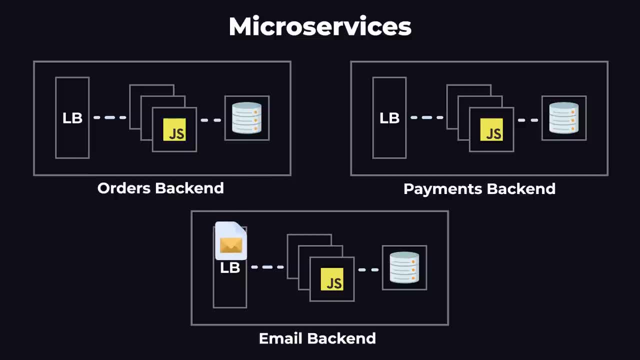 our orders backend will send a request to the email backend, which will send the email. So splitting up our backend into separate backends like this is called microservices, and it helps keep our codebase smaller and more focused. Each microservice does not have to use the same programming language and database. 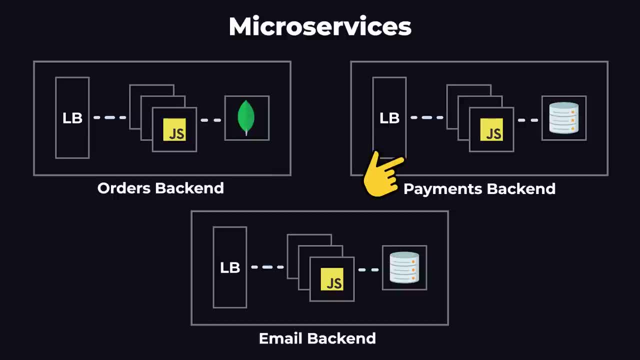 one microservice can be using JavaScript and MongoDB, while another microservice can be using Python and MySQL. Now, to make this even easier, there are companies out there, like Twilio, who have already created an email service, So Twilio provides a backend and an API for sending emails. 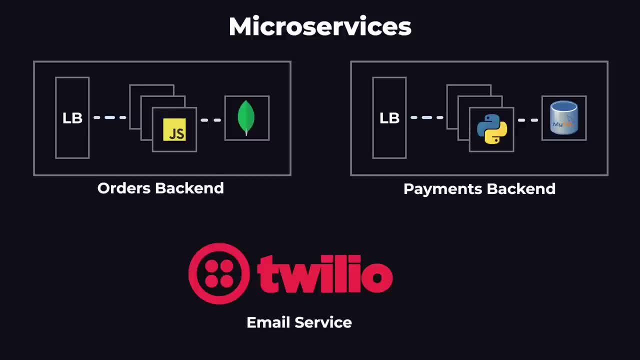 So, instead of us creating our own email microservice, our backend can just send requests to Twilio's backend. When a company provides a backend and an API that outside applications can use, this is called a service. When a company provides a backend and an API that outside applications can use, this is called a service. 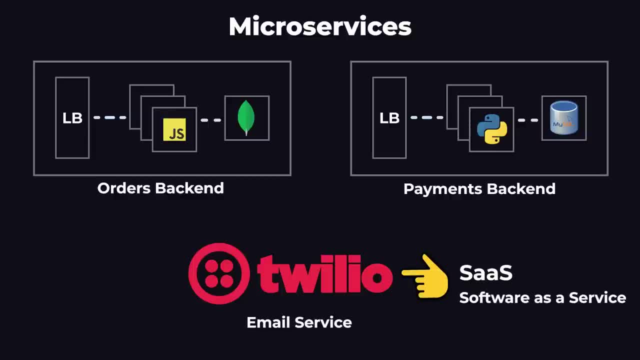 SaaS software as a service, Pretty much everything you do in the backend. that's complicated. there's probably a SaaS company out there that already provides that service and you can just use that service instead of building your own microservice. So these three concepts we just looked at. infrastructure as a service: 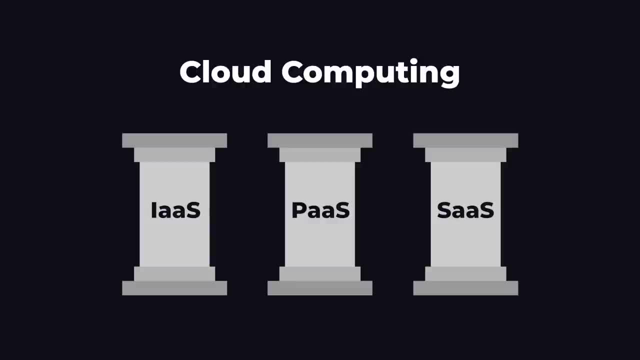 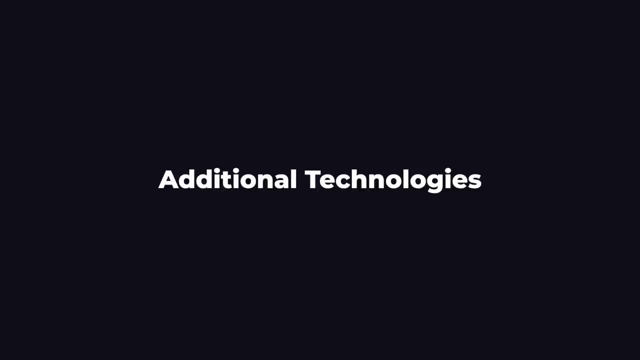 platforms as a service and software as a service are the three foundations of cloud computing. These days, most companies use cloud computing to run the backend for their websites instead of buying and managing physical services. In this last section, I want to introduce some additional technologies you might see. 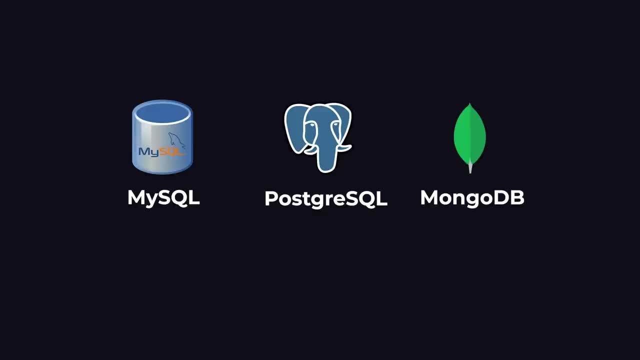 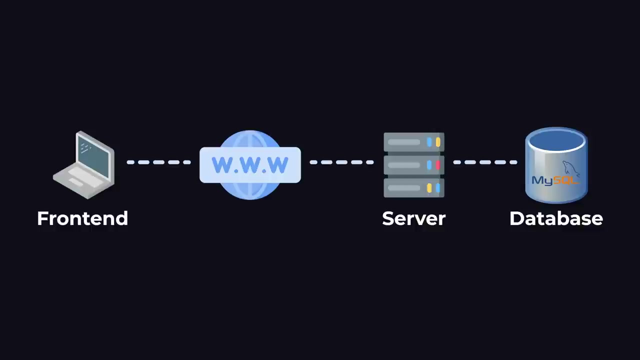 in the backend. Previously we mentioned the databases MySQL, Postgres and MongoDB. These are sometimes called primary databases because they're the main database that our website uses. Generally, we start our backend with a server and a primary database and then bring in these additional technologies if we need to. 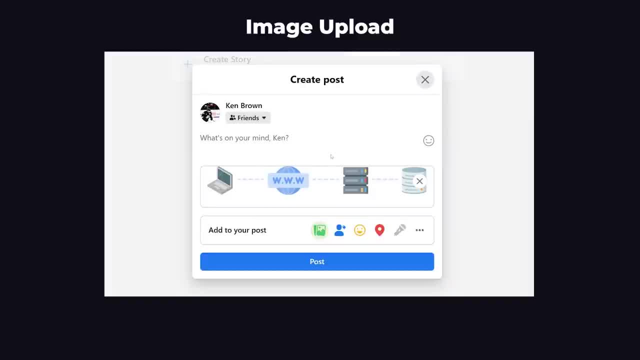 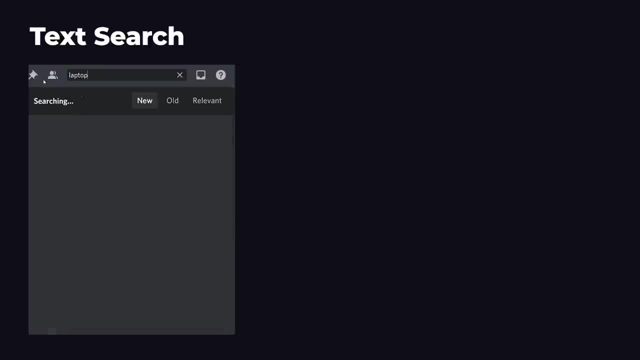 If we allow our users to upload images, a primary database is not good for storing images, so we would use a server, We would use a blob store like AWS S3, and a CDN like CloudFront to store and load user-uploaded images. If we want to allow text search, primary databases are very slow at text search. 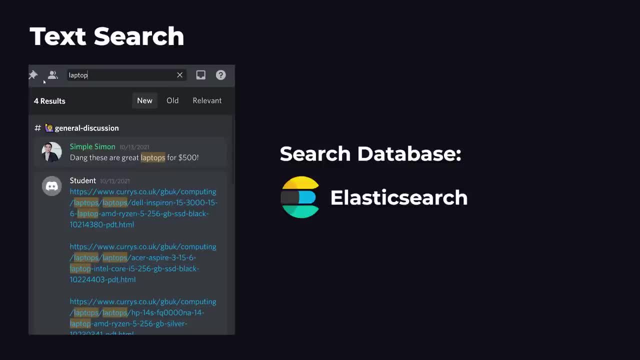 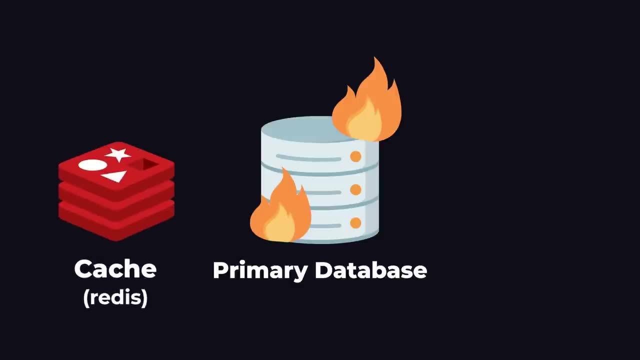 so we would bring in a search database like Elasticsearch. If our website is getting a lot of traffic and we need to take some stress off our primary database, we would add a cache like Redis to improve performance. If we want to do data science, 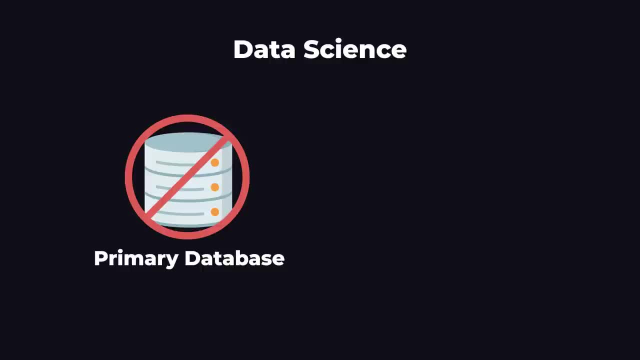 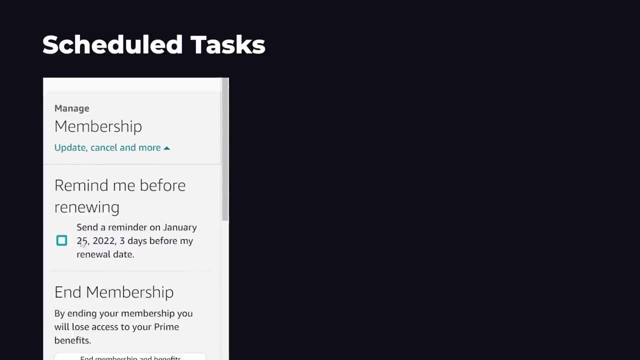 we don't want to do the data analysis, we would add a database like Snowflake to do the data analysis. If we want to schedule a task for later- for example, Amazon might want to email their users before their Amazon Prime subscription renews- we would use a job queue like RabbitMQ to schedule.